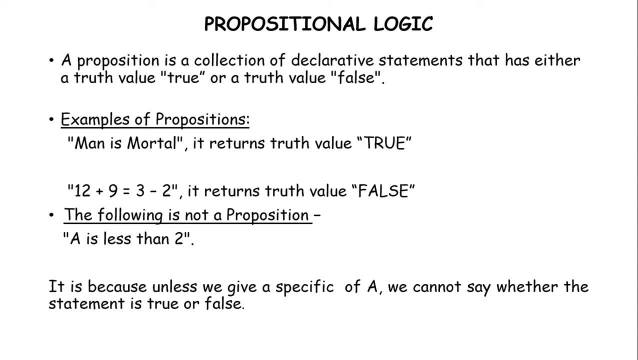 not equal to 1.. So 12 plus 9 is equal to 3 minus 2 is a proposition and the truth value that it will return is false. Why? Because 21 can never be equal to 1.. Now let us consider another statement. It says: 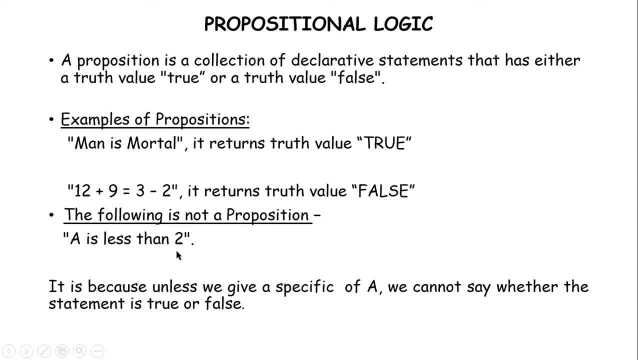 a is less than 2.. This is not a proposition. Why this is not a proposition? Because we do not know the value of a here. So unless we know the value of a, we cannot know the value of a. So unless we know the value of a, we cannot know the value of a. 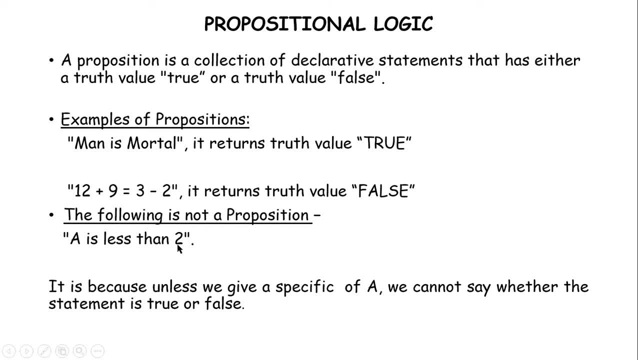 We cannot say whether it is less than 2 or not. If I do not know the value of a, I will not be able to decide, or I will not be able to come to the conclusion, whether a is less than 2 or not. So 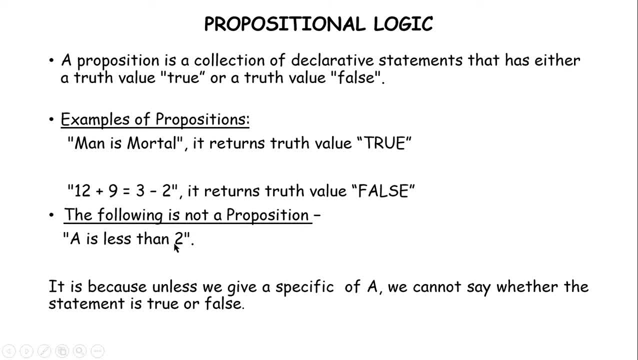 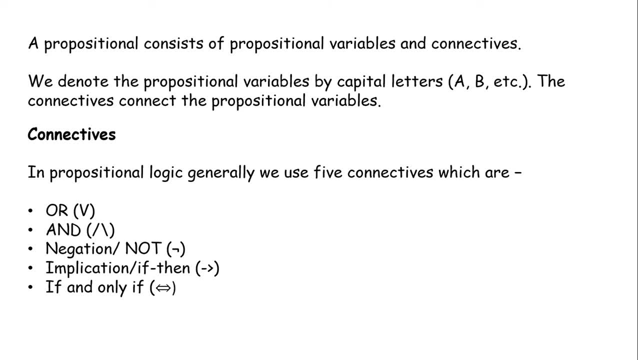 that means this is not a proposition. A proposition basically consists of propositional variables and connectives, A proposition which is a declarative statement. Any such declarative statement consists of two important elements. One is the propositional variable and the other is the. 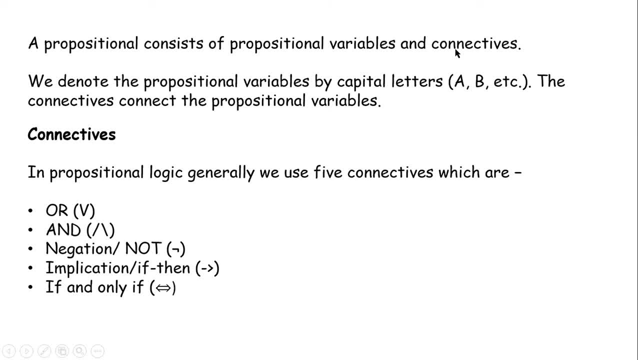 connectives. A propositional variable is related to the propositional variable. in a problem- solver Road- where the propositional variables are identical after a system of 가 and Rep, The propositional variables are linked to the propositional variables. The propositional variables plus the connective gives you what. 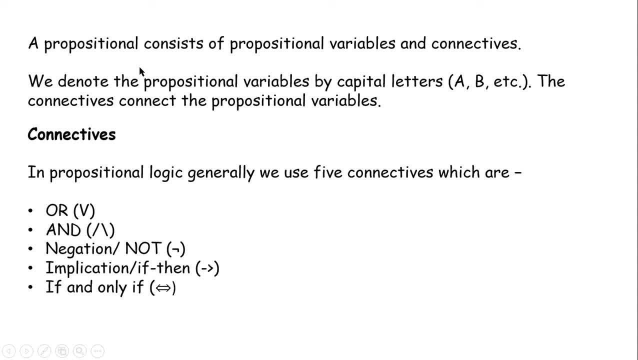 Gives you a propositional. Now let us see what connectives are. A connective is basically, as I told you, connect the propositional variables. So how many connectives do we have? We have five different types of connectives. 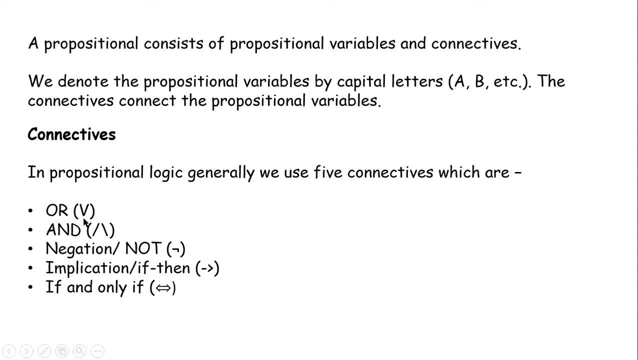 The OR connective. this is the symbol for the OR connective. Then we have the AND connective. this is the symbol for the AND connective. Then we have the negation or not connective. this is the symbol for the not connective. 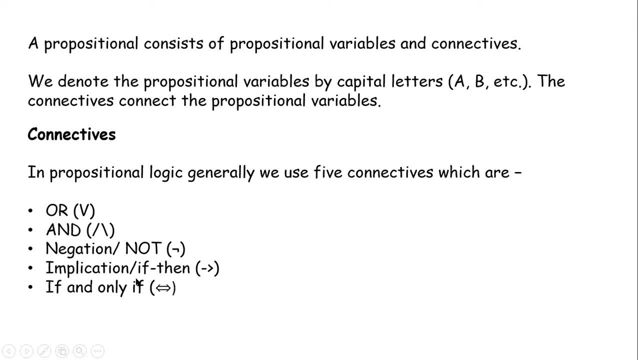 Then we have the implication or if-then connective. this is the symbol for the if-then or implication connective. And the last one, which is the if-and-only-if connective, and this is the symbol for the if-and-only-if connective. 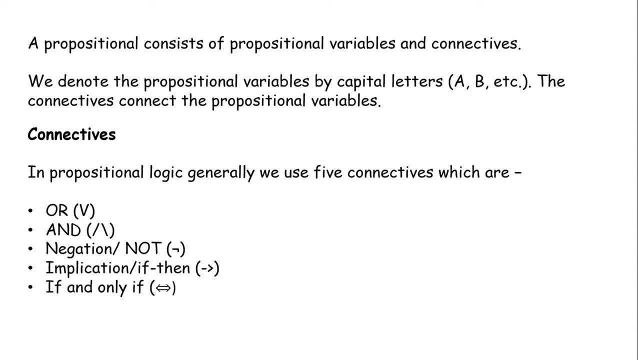 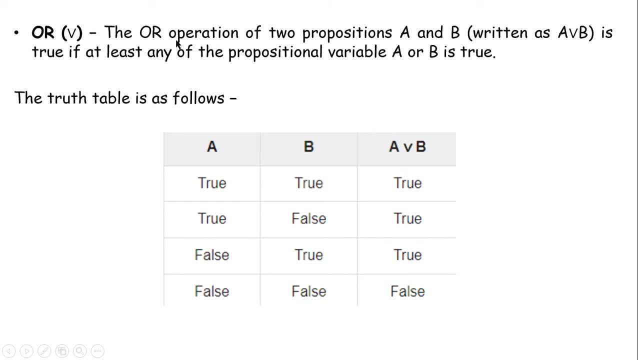 Now we will study all these five connectives in detail. First of all, we will start with the OR connective. The OR connective, The OR connective or the OR operation of two propositions. If I assume, I have two propositional variables, A and B. 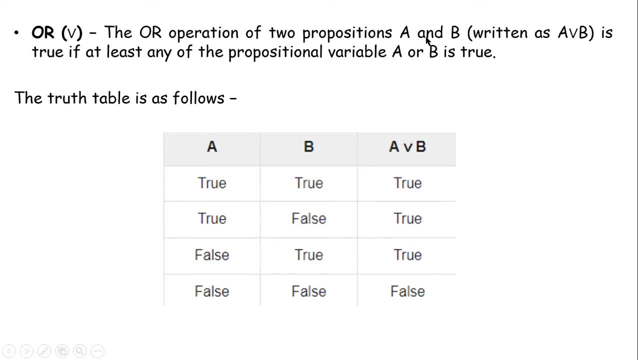 So the OR operation of these propositional variables A and B, which is written like this, using the OR symbol A or B, is true if at least any one of the propositional variable among A or B is true. That means the OR operation of the propositional variables A and A or B will be true if any either any one of them is true. 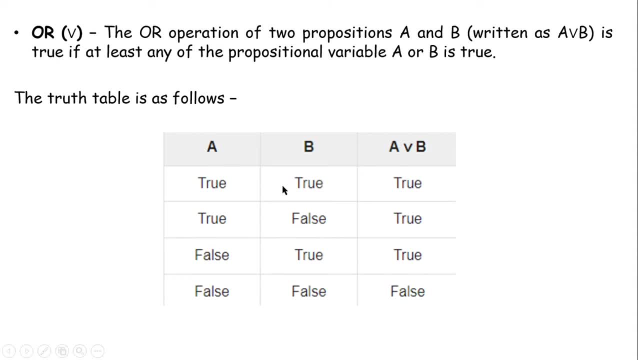 So either A is true or B is true. in that case A or B will be true. Here we can see. this is the truth table. that can help you better understand the OR operation or the OR connective. Now, if the value of A is true and the value of B is true, here A and B are both propositional variables. 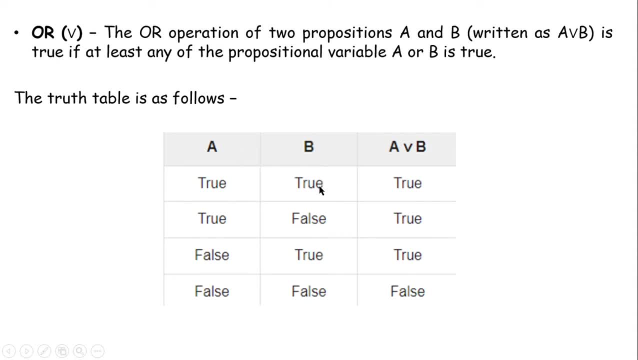 So if the value of A is true and the value of B is true, then obviously the value of A or B will also be true, because the condition here is that either one has to be true or the other one has to be true. In that case A or B will be true. but if here we are having both as true, then obviously A or B will be true. 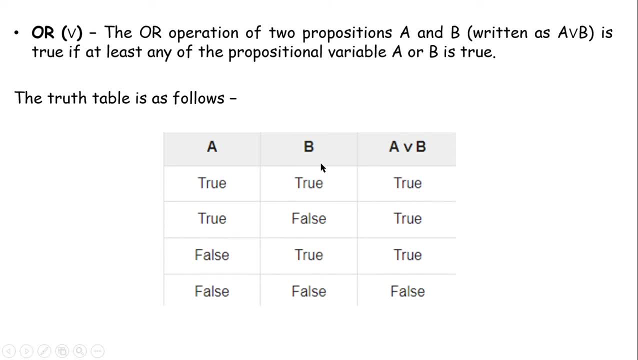 Moving on. if A is true and B is false, even in that case A or B will be true, because either one of the variable has to be true, and here A is true. Then if A is false and B is true, again in that case A or B will be true, because either A has to be true or B has to be true. 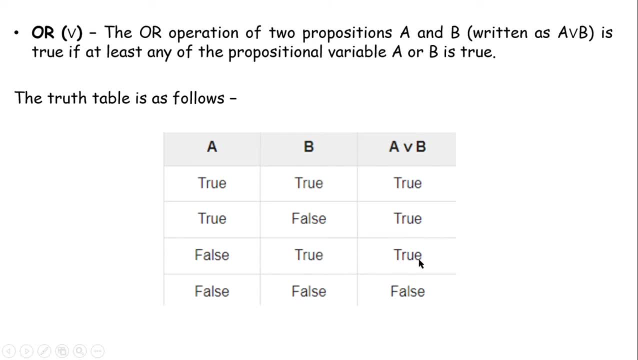 So here B is true. So in that case A or B will be true. Then if A is false and B is also false, in that case A or B will be false, because at least one of the variable has to be true for A or B to be true. 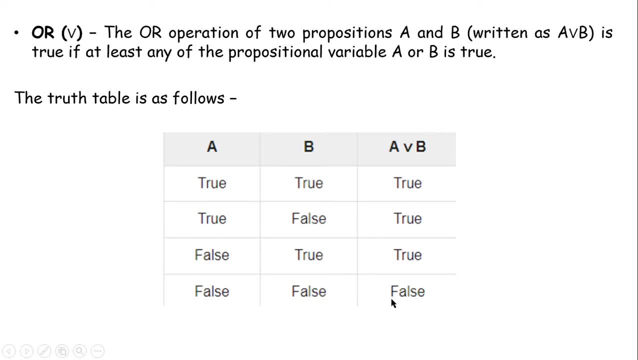 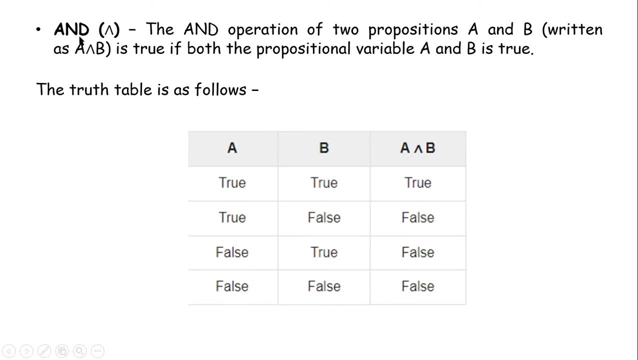 So here we can see both A and B are false. So A or B is also false. Then the next connective is the AND operation. Now the AND operation on the propositional variables. again we will take these two variables named as A and B. 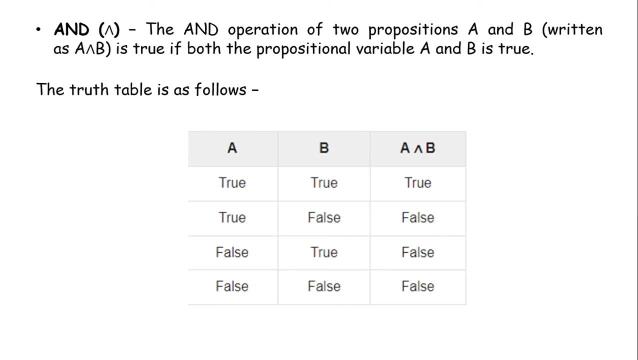 So the AND operation, So the AND operation on the propositional variables. again we will take these two variables, named as A and B, AND operation on the propositional variables A and B, which is written by this symbol: A and B is true if both A and B are true. So the connective itself specifies the operation that. 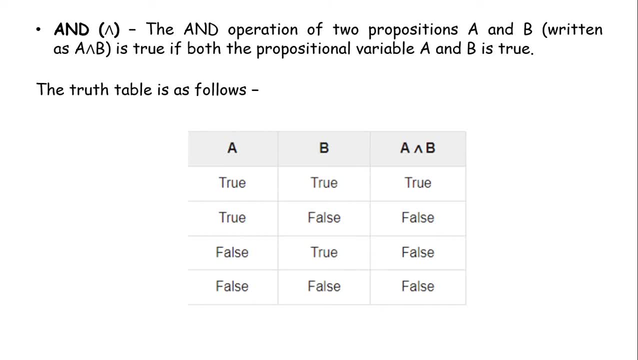 AND. the AND operation is being done on A and B. So that means if both A and B will be true, only then the result of the operation will also be true. So if there is a propositional variable A and there is a propositional variable B, then in that case, if A is true and B is true, then A and 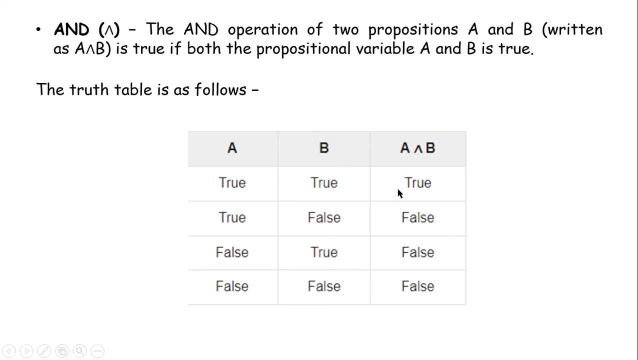 B will be true because both A and B are true. Now, if A is true and B is false, then A and B will be false because both A and B are not true here. Here, B is false Again, if A is false and B is true. 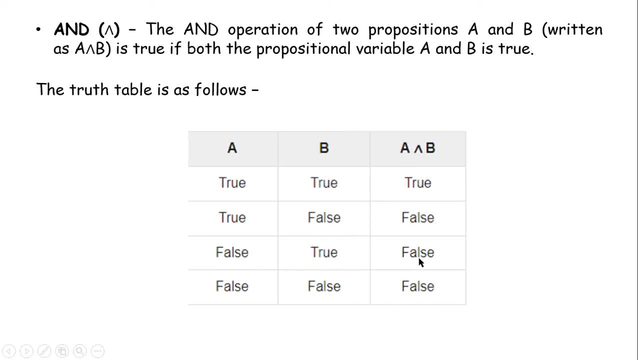 then A and B will be false. Why? Because both A and B are not true here. Here A is false, Then A and B are not true. Here A and B are not true. Here A and B are not true. Here A and B are not. 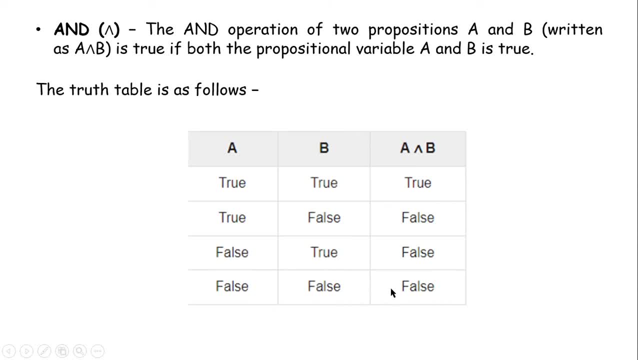 true. If A is false and B is also false, then obviously A and B will be false, because A and B are both false. So for the result of the operation A and B to be true, both the variables A and B have to be true. So here in the truth table you can see that only for this row we have a true value. 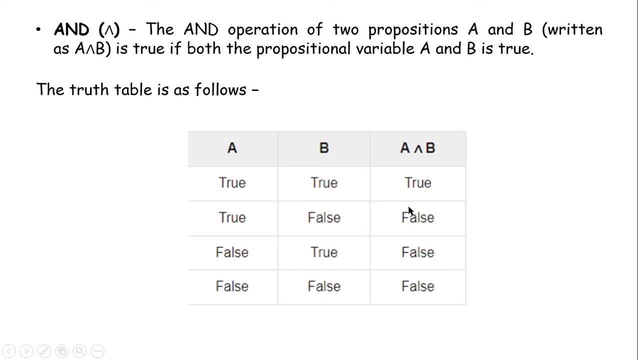 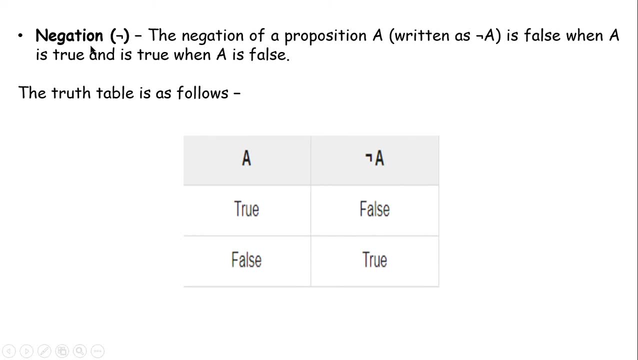 truth value true for A and B. rest for all of the rows we have the truth value false. Next is the negation operation. So the negation of a proposition- A is written by this symbol- is false when A is true and is true when A is false. So in other words, I can say that if A is true, the negation of A will be its opposite. 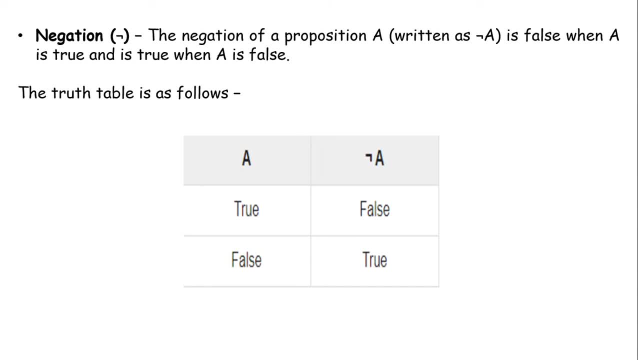 that is false. and when A is false, the negation of A will be its opposite. that is true. So for the negation operation you do not need two variables. The negation operation can be done on a single variable. So here, if A is true, then A negate negation A will be false, and if A is false, then negation A will. 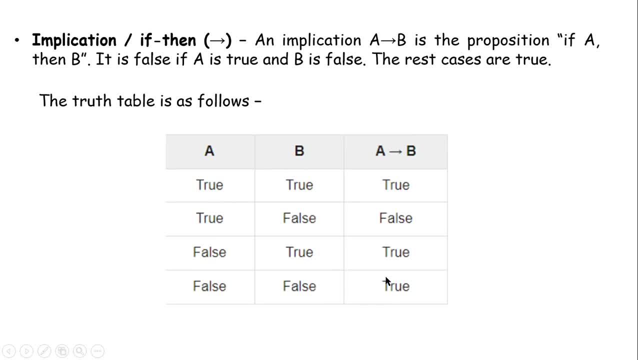 be true. Next is the implication or the if, then connective. This is the symbol. this arrow is the symbol for the implication or the if then connective. So an implication that means A implies B is the proposition that if A, then connective. 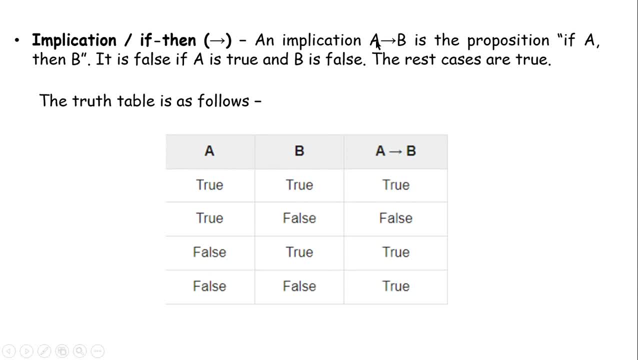 It is read as the implication symbol for A implies B is read as if A then B. It is false if A is true and B is false. So if A is true, if the truth value of A is true and the truth value of B is false, 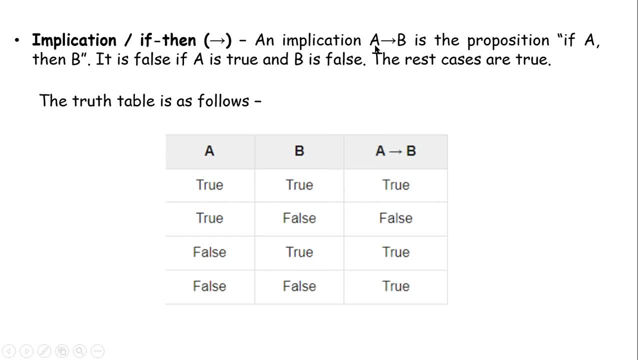 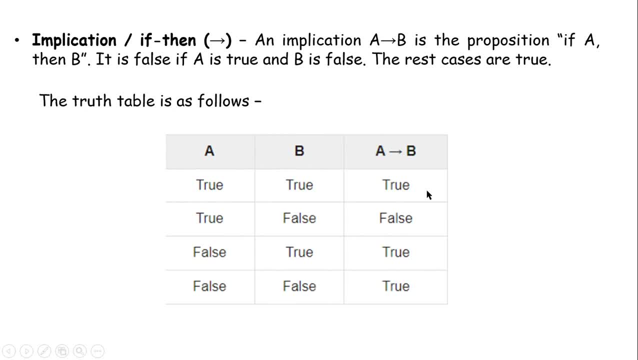 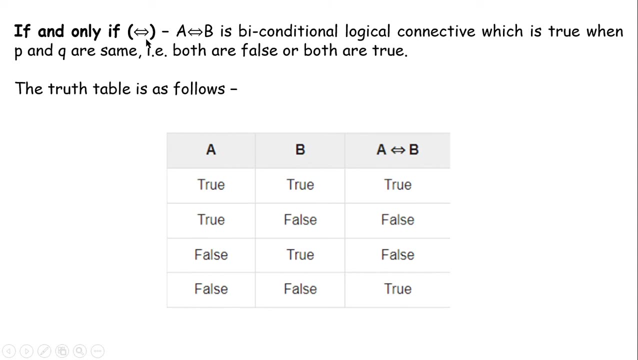 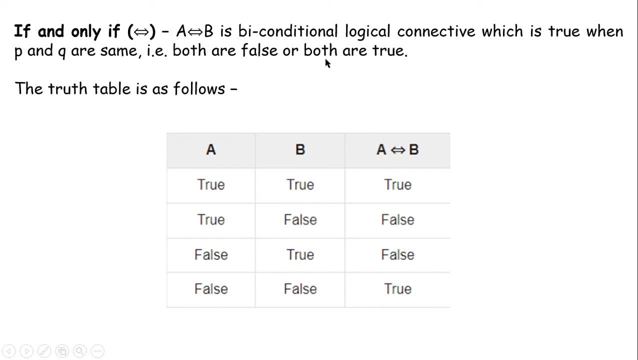 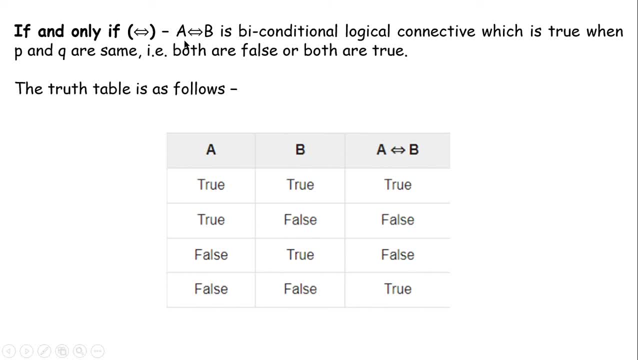 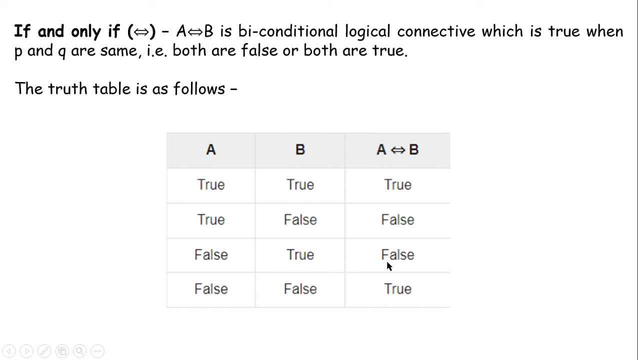 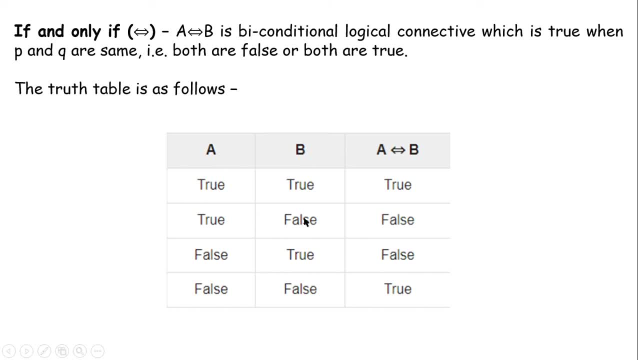